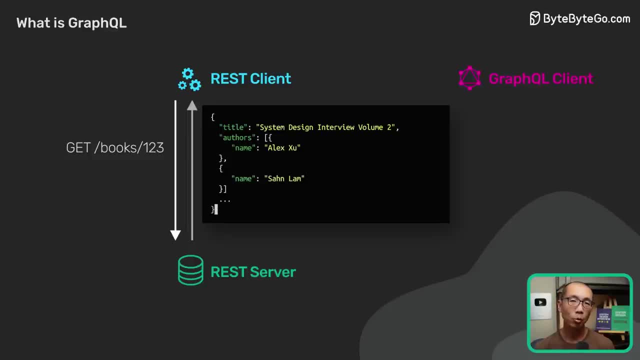 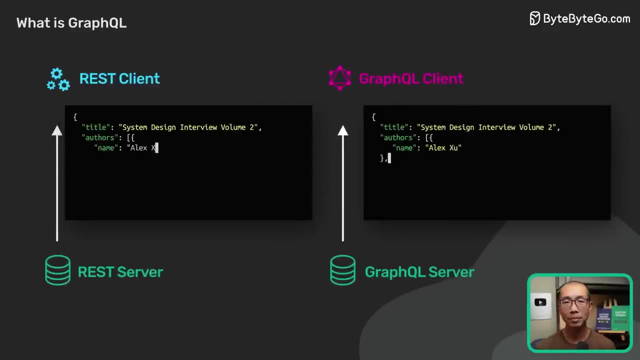 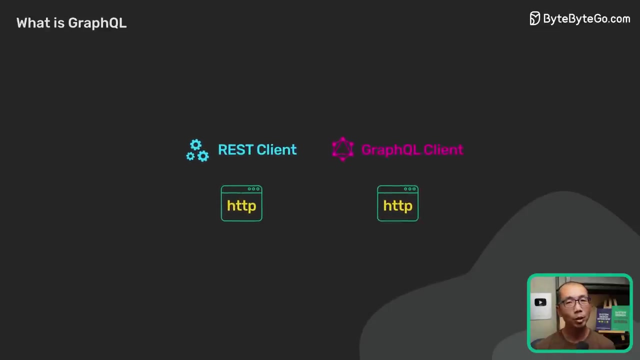 GraphQL. Now, to do that, we need to define a query like this. Now we can send a request to the GraphQL endpoints to fetch the same data. As we can see, REST and GraphQL both use HTTP, Both make a request via a URL and both can return a JSON response in the same shape. 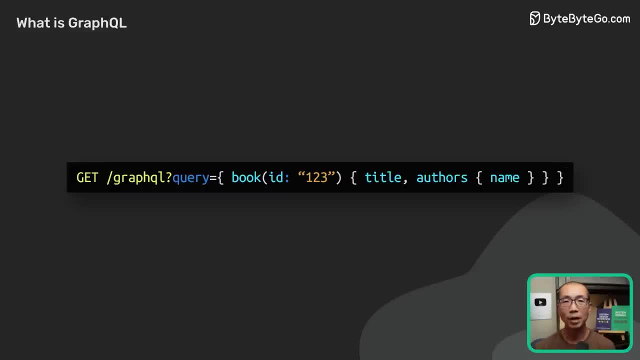 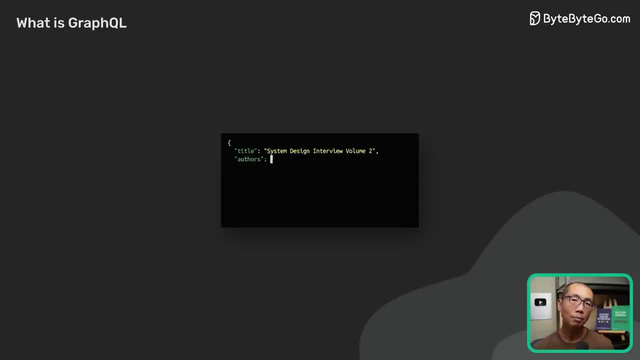 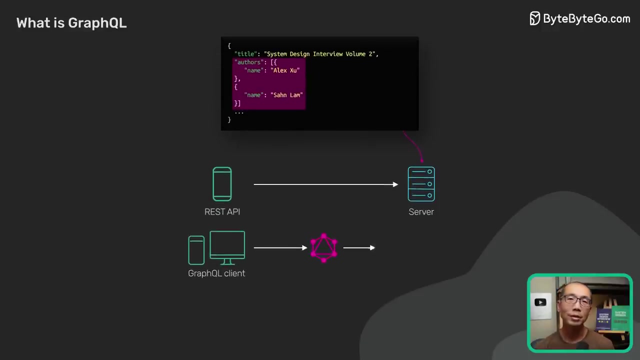 Here are the differences. With GraphQL, we specify the exact resources we want and also the fields we want. In the REST example, the API implementer decided for us that authors are included as related resources. With GraphQL, the client decides what to include. 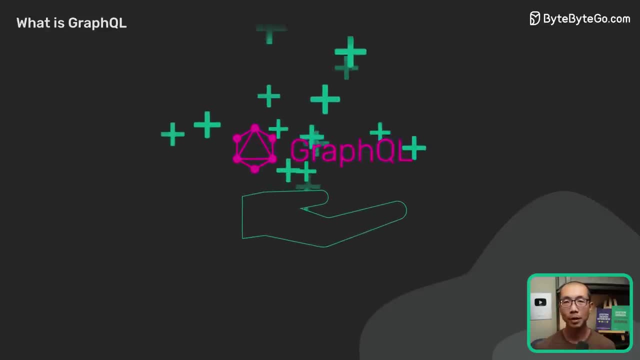 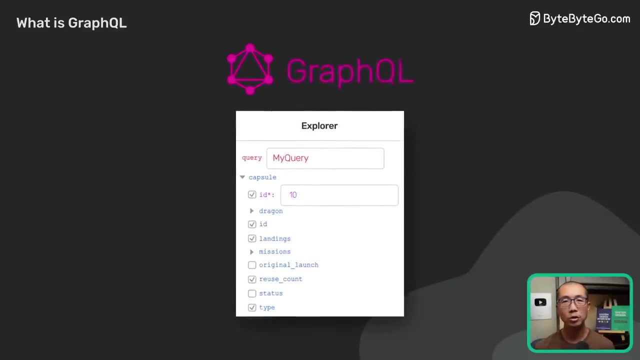 This brings up one of the main benefits of GraphQL. GraphQL doesn't use URLs to specify the resources that are available in the API. Instead, it uses a GraphQL schema. We can send a complex query that fetches additional data according to the relationships defined in the schema. Doing the same in REST is more complicated. 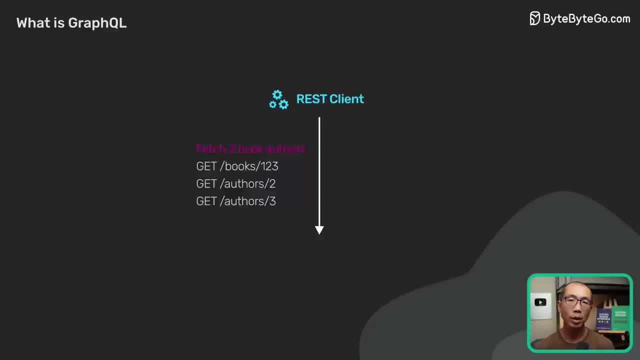 We would have to do that client-side with multiple requests. This is a common problem, resulting in N plus one queries. Next, let's discuss some drawbacks. The beauty of REST is that we don't need special libraries to consume someone else's API. 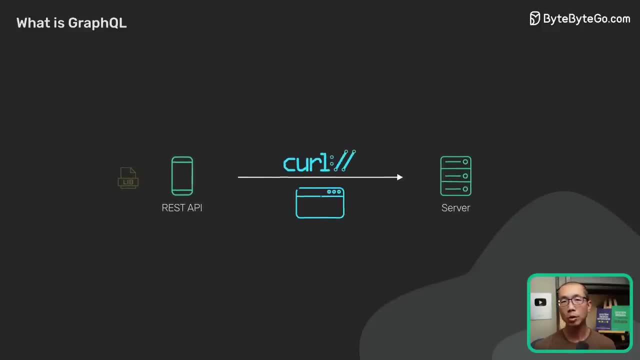 Requests can simply be sent using common tools like cURL or simply a web browser. In contrast, GraphQL requires heavier tooling support, both on the client and server size. This requires a sizable upfront investment. This upfront cost might not be worth it, especially for 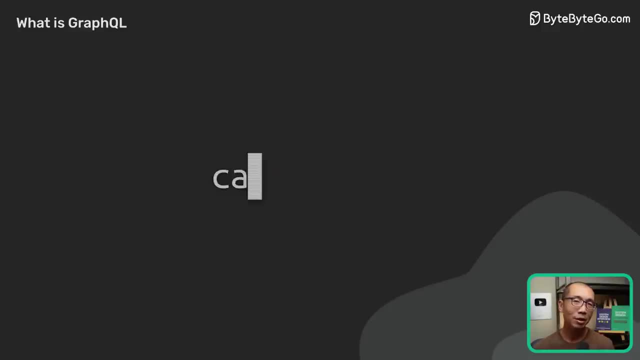 very simple CRUD APIs. For example, if we want to use GraphQL as a tool, we need to use GraphQL as a tool. Another criticism of GraphQL is that it is more difficult to cache. REST uses HTTP GET for fetching resources and HTTP GET has a well-defined caching behavior. 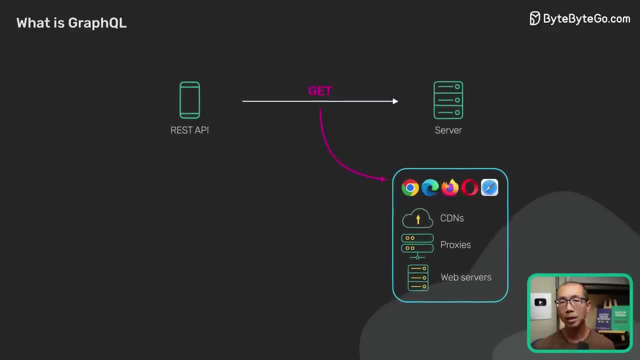 that is leveraged by browsers, CDNs, proxies and web servers. GraphQL has a single point of entry and uses HTTP POST by default. This prevents the full use of HTTP caching. With care, GraphQL could be configured to better leverage HTTP caching. The detail is very nuanced For this video.